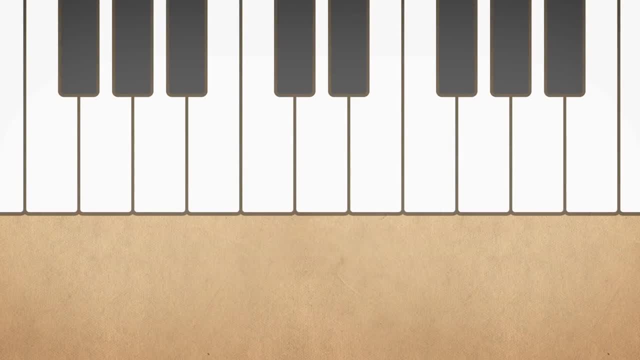 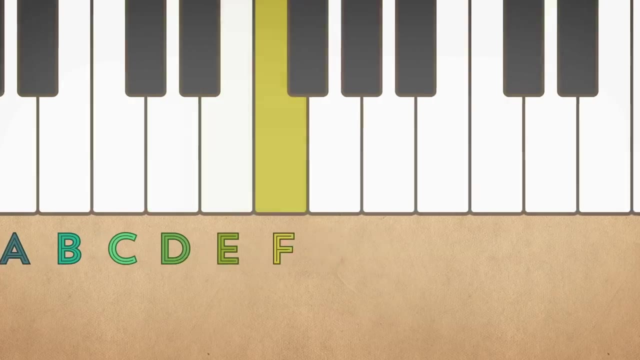 pretty much any instrument you can think of. In the Western music tradition, pitches are named after the first seven letters of the alphabet: A, B, C, D, E, F and G. After that the cycle repeats itself: A, B, C, D, E, F, G. A, B, C, D, E, F, G, and so on. But how do these pitches get their? 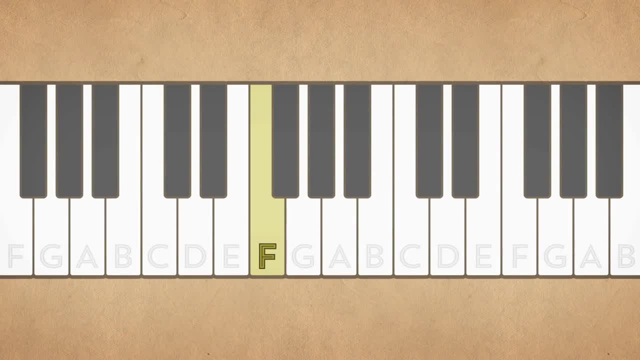 names. Well, for example, if you played an F and then played another F, higher or lower on the piano, you'd notice that they sound pretty similar compared to, say, a- B. Going back to the staff, every line and every space between two lines represents a separate pitch. 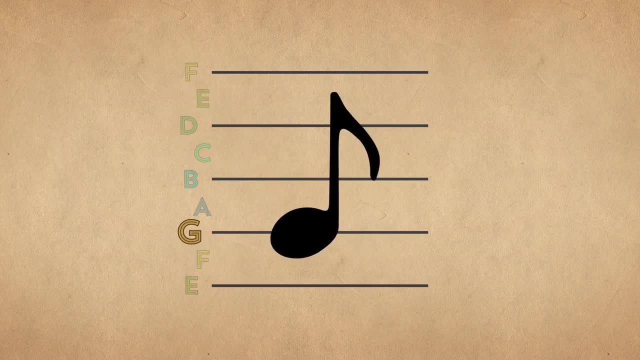 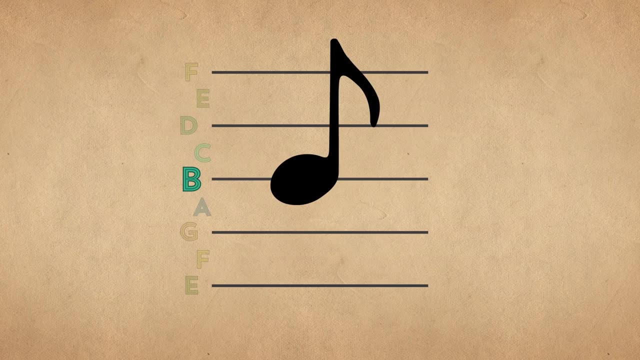 If we put a note in one of these lines or in one of these spaces, we're telling a performer to play that pitch. The higher up on the staff a note is placed, the higher the pitch. But there are obviously many, many more pitches than the nine that these lines and spaces. 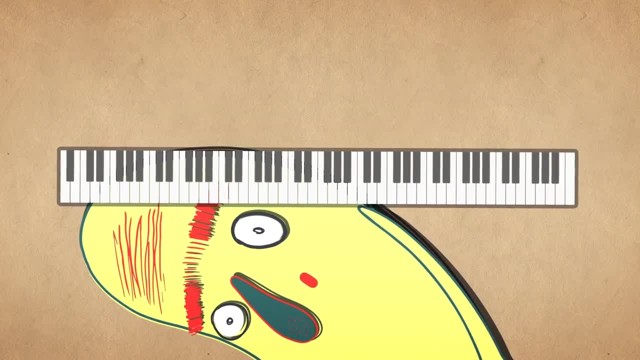 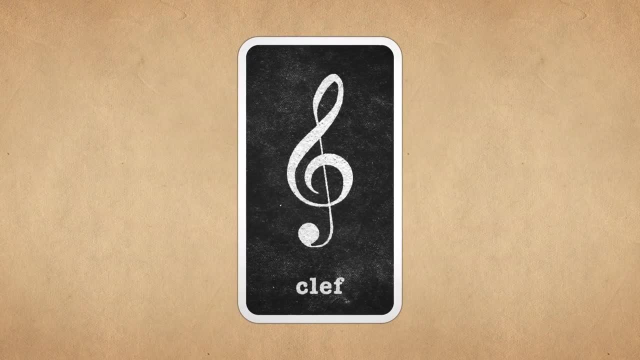 give us A grand piano, for example, can play 88 separate notes. So how do we condense 88 notes onto a single staff? We use something called a clef. A clef is a weird-looking figure placed at the very beginning of the staff and it acts. 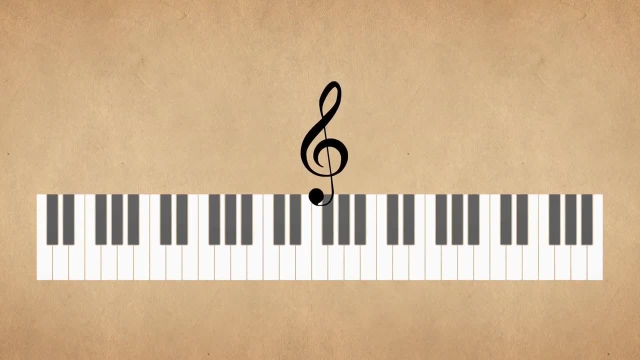 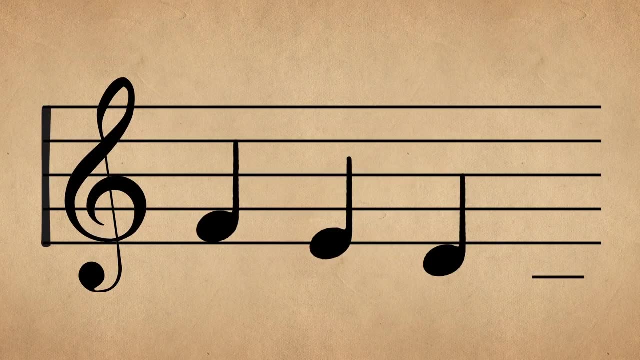 like a reference point telling you that a particular line or space corresponds to a specific note on your instrument. If we want to play notes that aren't on the staff, we kind of cheat and draw extra little lines called ledger lines and place the notes on them. 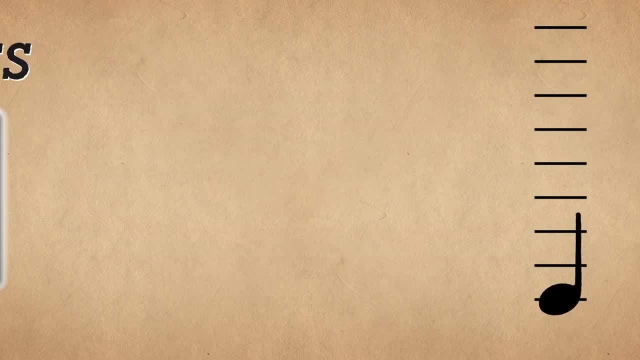 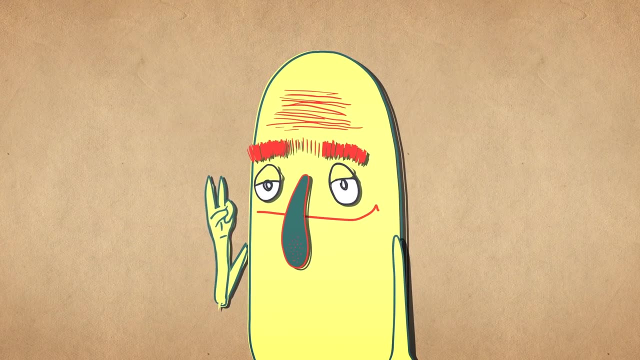 If we have to draw so many ledger lines that it gets confusing, then we need to change to a different clef. As for telling a performer when to play the notes, two main elements control this: The beat and the rhythm. The beat of a piece of music is by itself kind of boring. 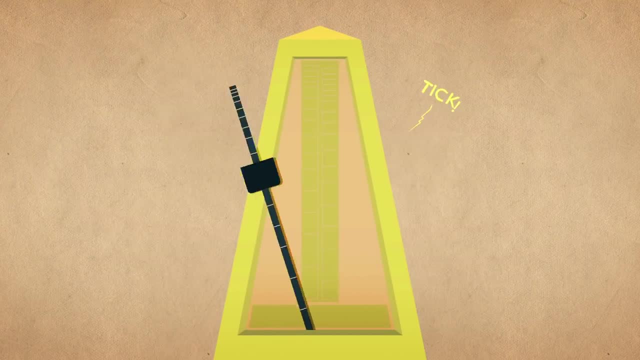 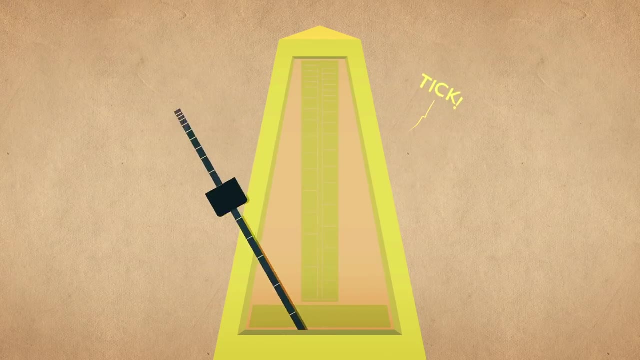 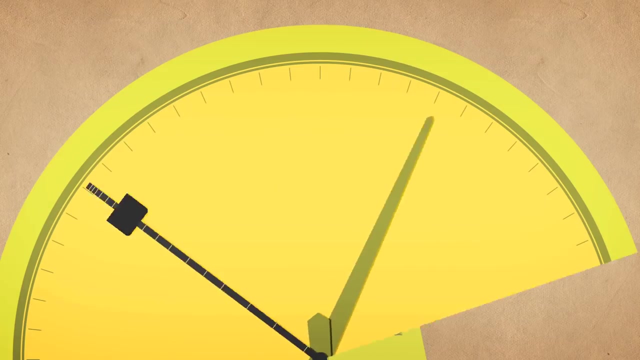 It sounds like this. Notice that it doesn't change. It just plods along quite happily. It can go slow or fast or whatever you like. really, The point is that, just like the second hand on a clock divides one minute into 60 seconds. 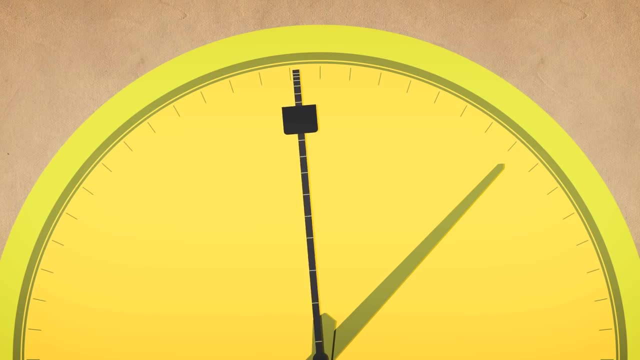 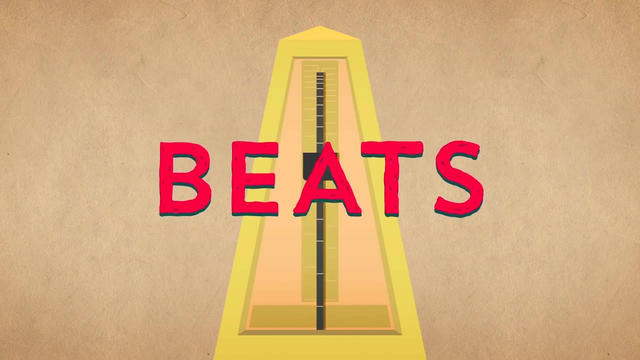 with each second just as long as every other second. the beat divides a piece of music into little fragments of time that are all the same length: Beats. With a steady beat as a foundation, we can start adding rhythm to our pitches, and that's. 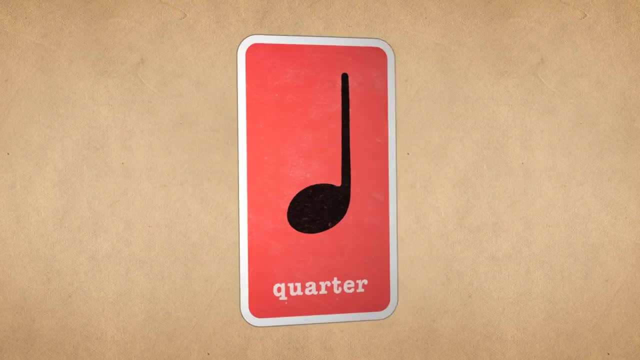 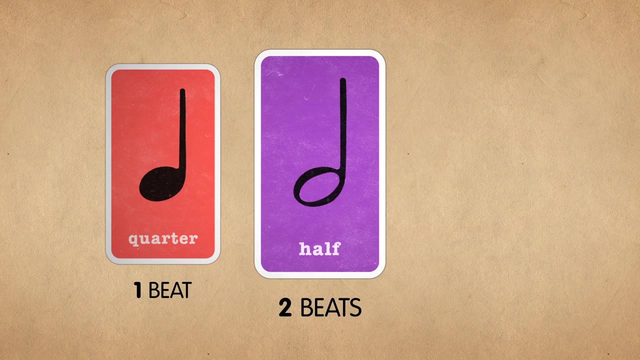 when music really starts to happen. This is a quarter note. It's the most basic unit of rhythm and it's worth one beat. This is a half note and it's worth two beats. This whole note here is worth four beats, and these little guys are eighth notes worth. 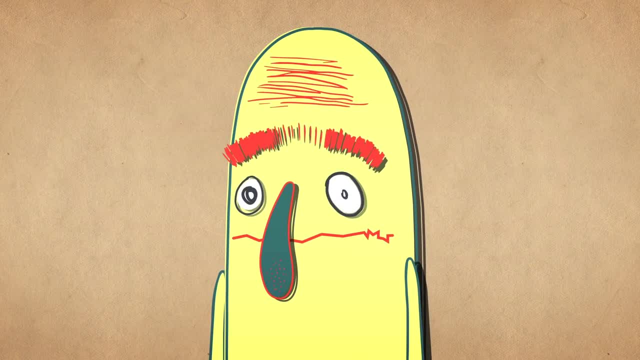 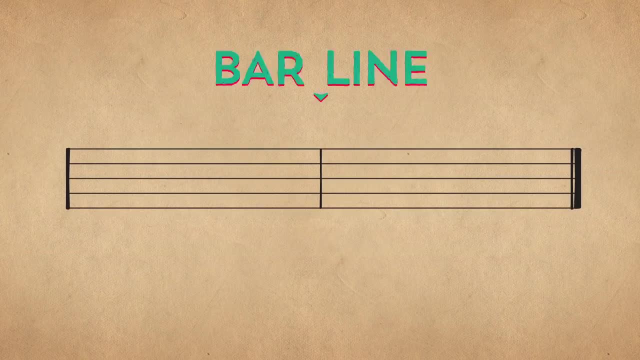 half a beat each Great you say. What does that mean? You might have noticed that across the length of a staff there are little lines dividing it into small sections. These are bar lines and we refer to each section as a bar. 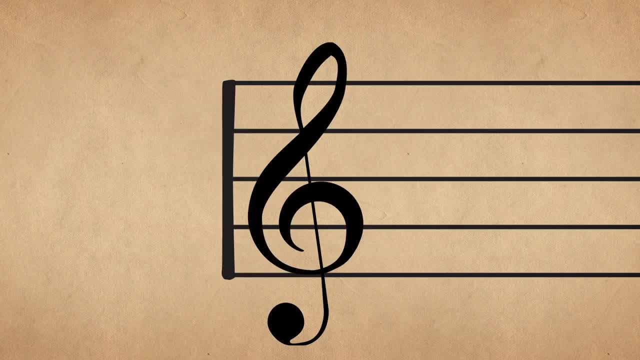 At the beginning of a piece of music, just after the clef, is something called a bar. This is a bar. This is a bar. This is called the time signature, which tells the performer how many beats are in each bar. This says there are two beats in each bar. 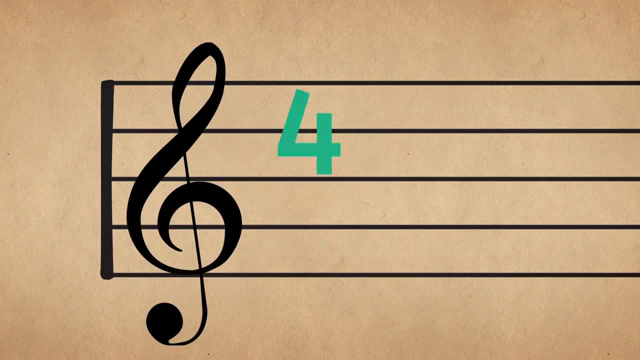 This says there are three, This one, four, And so on. The bottom number tells us what kind of note is to be used as the basic unit for the beat. One corresponds to a whole note two to a half, note four to a quarter, note an eighth. 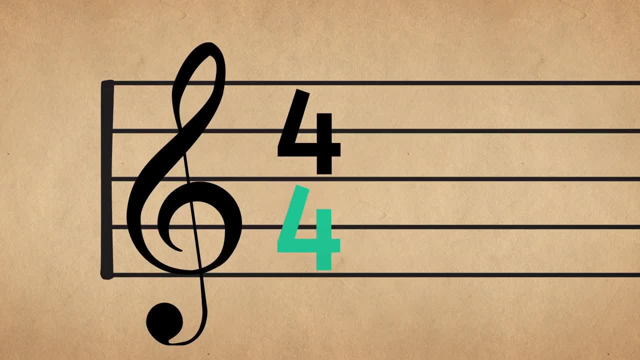 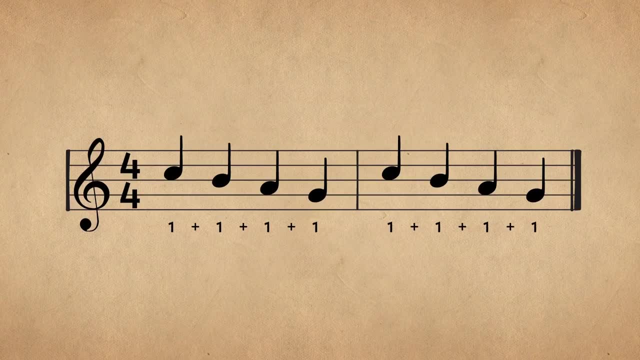 to an eighth note and so on. So this time signature here tells us that there are four quarter notes in each bar: One, two, three, four, One two, three, four, B4 and so on. But like I said before, if we just stick to the beat it gets kind of boring. 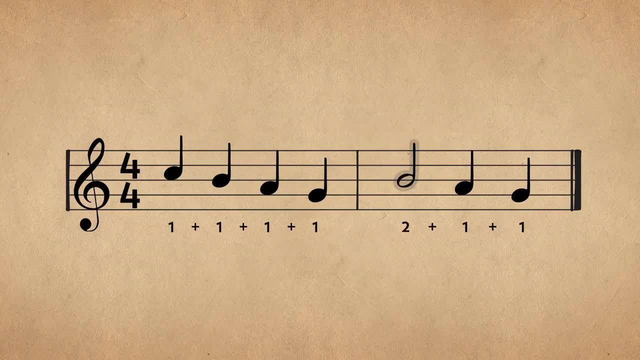 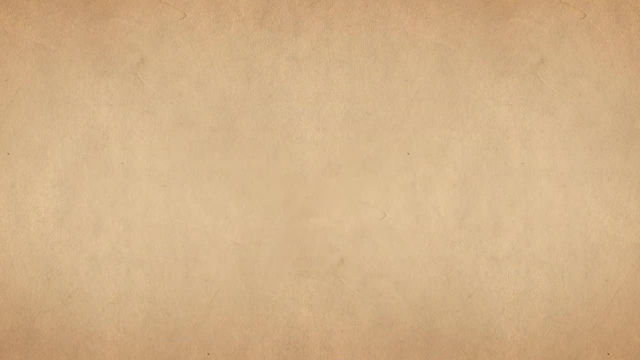 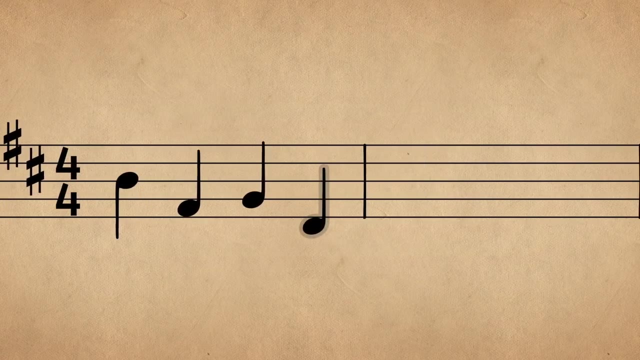 so we'll replace some quarter notes with different rhythms. Notice that even though the number of notes in each bar has changed, the total number of beats in each bar hasn't. So what does our musical creation sound like? Sounds okay, but maybe a bit thin. right, Let's add another instrument with its own. 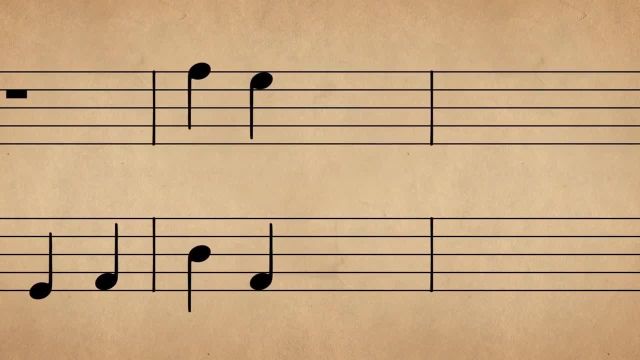 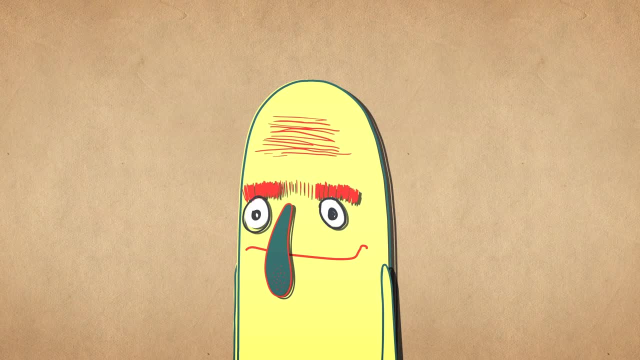 rhythm. Now it's sounding like music. Sure, it takes some practice to get used to reading it quickly and playing what we see on our instrument, but with a bit of time and patience you could be the next Beethoven Or Justin Bieber. Yeah, We'll have to see if it's going to work. There's a lot of different ways you can build the weaving. There are so many different ways to add things Like, for example, with the violin, you can't add all of the notes in the same time. but then when you add notes in the next bar, the notes will be perfectly symmetrical, so it gets a little bit more natural, right? Exactly, If we had shown this format before, we'd have moved a step back and did this movement a couple of times and then we'd have used some of these notes. but if we'd moved the notes. we'd have added a few notes here and there. Then the notes would change, So it wouldn't really feel like something we would be doing. But that's what I mean. D line in Ensemble. Right now the music is perfectly symmetrical. 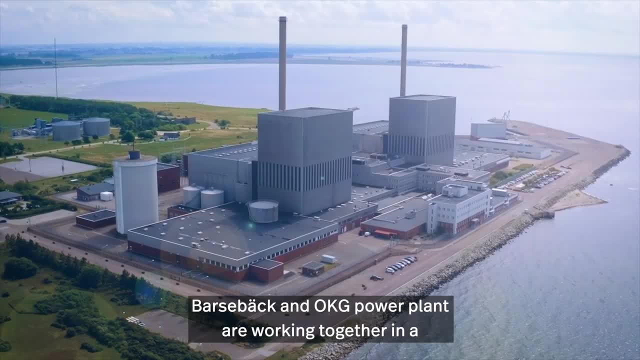 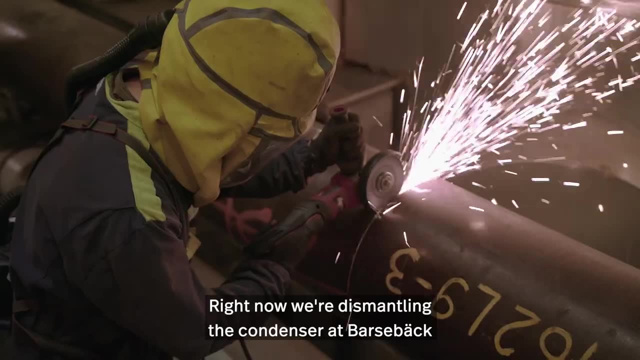 Barsebäck and OKG Power Plant are working together in a world-unique project where we take down the stations one by one in sequence. Right now we are dismantling the condenser at Barsebäck Power Station, Unit 1 and 2..